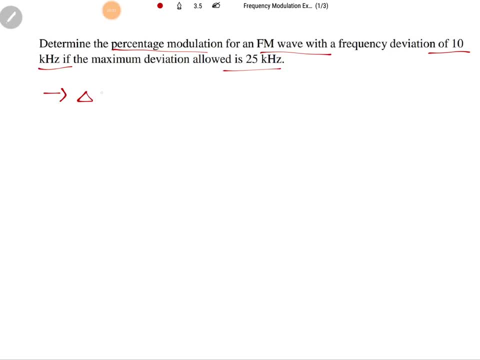 So here it have been given frequency deviation, delta F that is 10 kHz and maximum allowed deviation that is given by 25 kHz. So we are dealing with to calculate percentage modulation. So here we are dealing with to calculate percentage modulation of FM that is given by actual deviation divided by maximum allowed deviation into 100. 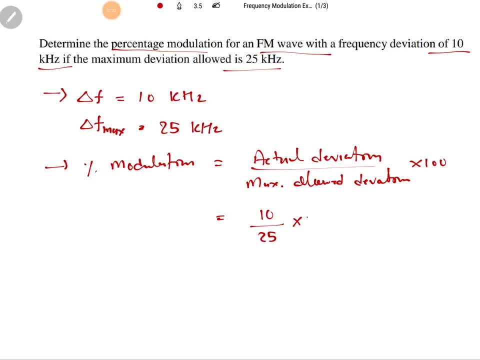 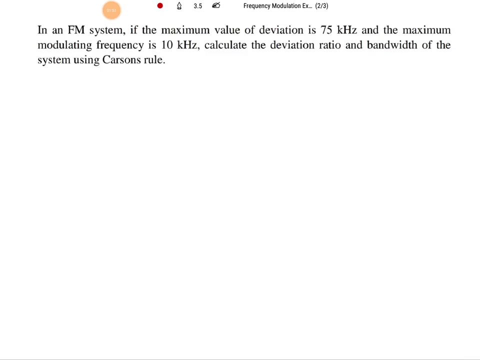 Maximum allowed deviation, that is 25 kHz into 100. So if you calculate this you will be finding it is 40 percentage. So percentage modulation is actual deviation divided by maximum allowed deviation. Now let us move on to next example. Now see in this question, in FM system if the maximum value of deviation is 10 kHz. 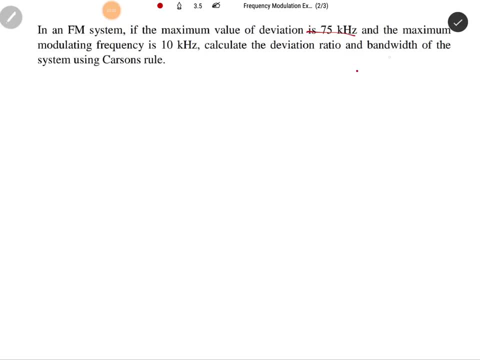 So here the maximum modulation is 75 kHz And the maximum modulating frequency, that is 10kHz. Then calculate deviation ratio and bandwidth of system using Carnot's rules. So here it has been given: maximum modulating frequency is given by 10 kilohertz and maximum value of deviation that is given by 75. 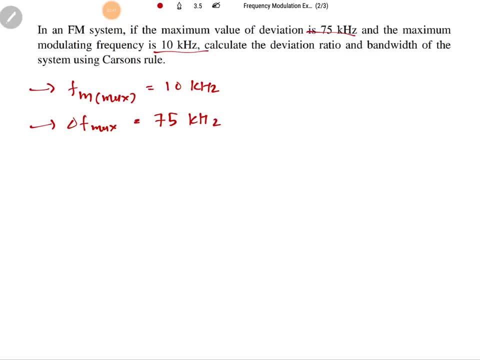 kilohertz. so first we will be calculating deviation ratio. so deviation ratio, that is Delta F max divided by FM max. so that will result into 75 kilohertz divided by 10 kilohertz. so deviation max, maximum deviation ratio, that will be 7.5. 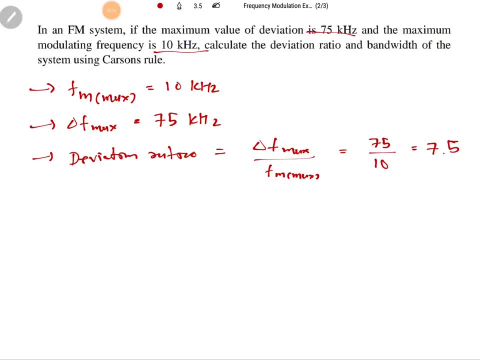 now we are delivered to calculate bandwidth using Carnot rule. so when we talk about bandwidth, system bandwidth by Carnot's rule that we can identify by 2 into FM max maximum modulating frequency plus deviation. so that is how we calculate system bandwidth by Carnot's rule. now here FM. 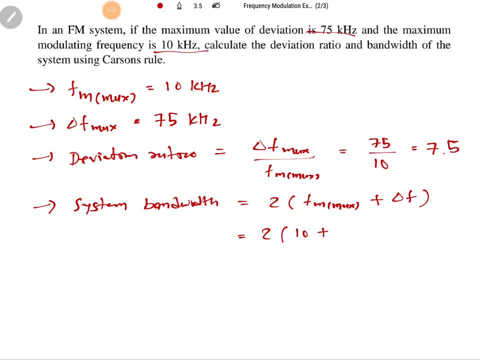 fm max, that is 10 kilo Hertz, plus Delta F, that is 75 kilohertz. so this is two into 85. it means it will be 170 kilohertz. so this will be system bandwidth as per carnot's rule. now let us move on to next example here, equation. 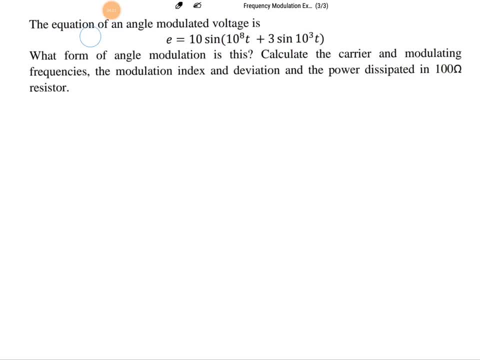 of angle modulation is given with fm max, which is 12XT of C per unit value, plus 505어나 151 one這個方式的旋律: bowel accuracy is a single那這樣的手段, Die aus 180airs per kulis Misvenchung, EU, вот這些例 covenant is a single Nebel. 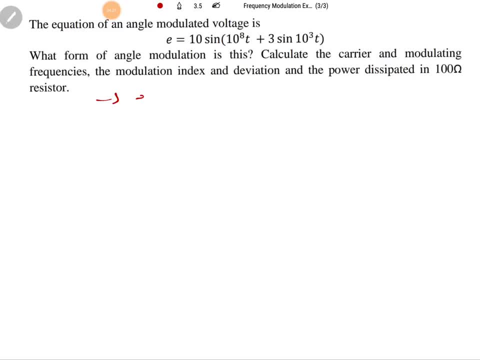 and that equation is: e is equals to 10 sine 10 to the power 8 t plus 3 into sine 10 to the power 3 t. and here we are delivered to calculate angle modulation. what is the form of angle modulation? calculate carrier and modulating. 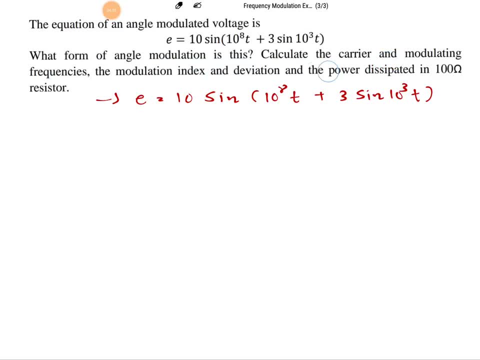 frequencies, modulation index, deviation power dissipated in 100 ohm resistor. so before we calculate all those things, let us compare this equation with standard form. so standard form of fm that is given by e is equals to e, c, e, sine omega c t plus m f. that is modulating index of fm into sine omega m t. so from this, 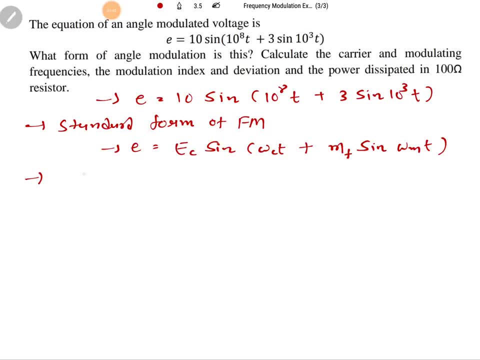 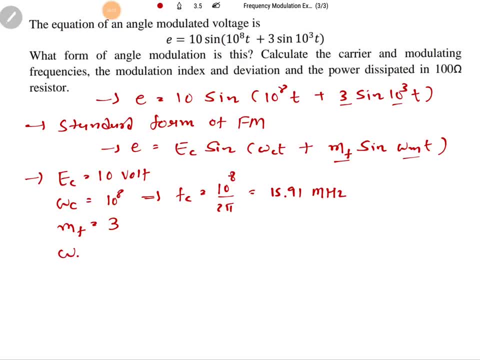 so these many things we can directly calculate from this now modulation index, mf, that is 3 and that even we can identify by Δf, by Fm. so we can calculate Δf and that is mf into Fm. mf is given by 3. 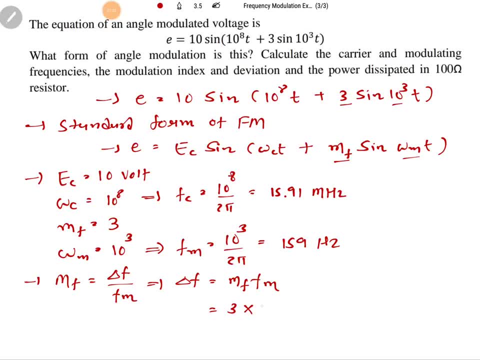 into Fm, So FM that is 159.. So we can identify deviation. that is 477 Hertz. Now here the last question, that is, power dissipated through 100 ohm resistor. That is what we are delivered to identify. 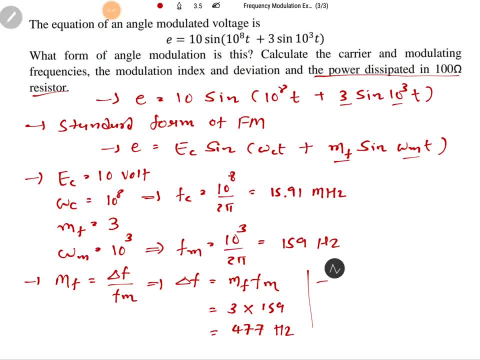 Okay, Now when we talk about power calculation, then power is P is equals to EC square divided by 2R, Where, by comparing this standard form with this given equation, we have calculated EC, that is 10 voltage. So 10 square divided by 2 into R, that is 100.